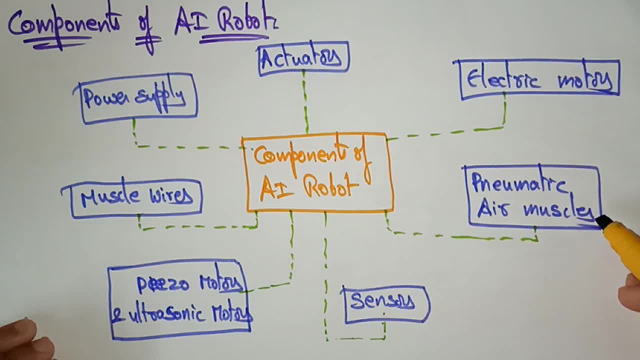 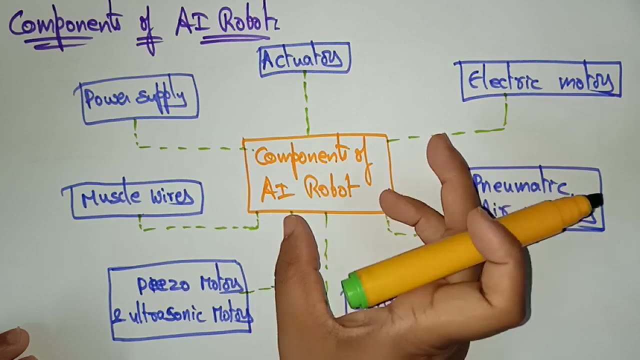 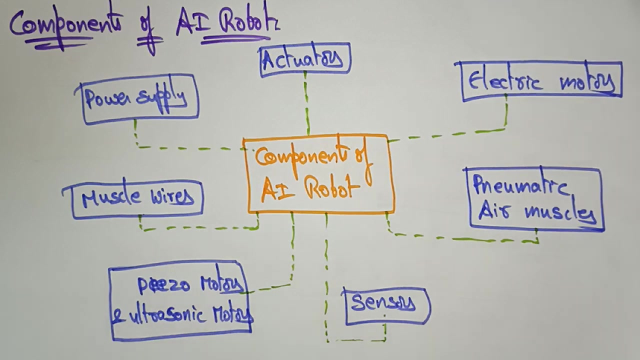 electric motors, pneumatic air muscles, sensors, ultrasonic motors, muzzle wires and the power supply. So these are all the different components that are used in the artificial intelligent robots. So with the help of all these components, only the robot is going to perform and manipulate the things. okay, It can do, it can act like a 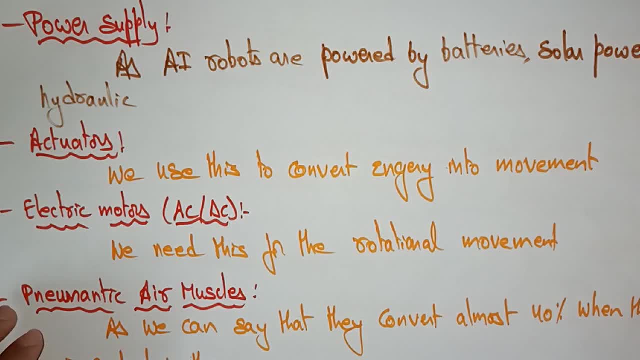 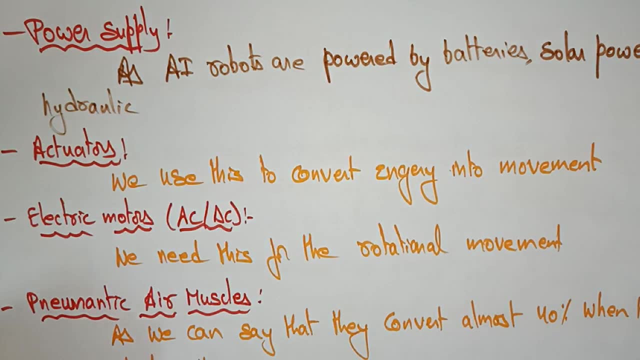 human, okay, and it is working on the real-time environment. Let's see, one by one, what is the components that we used in the artificial intelligent robot. The first thing is let's take the power supply. So the power supply is very important if the robot wants to work. 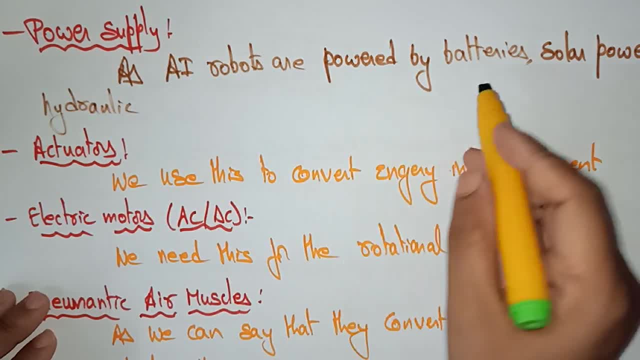 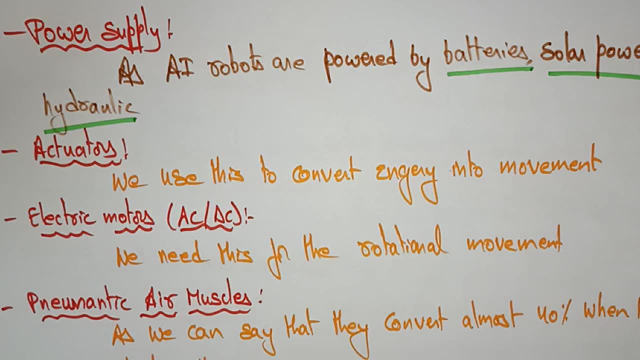 So as artificial intelligent robots are powered by batteries, solar power and even the hydraulic powers also. So these are the different ways that techniques that used for the power, giving the power supply to the robot, So you can power the robots by the help of batteries. 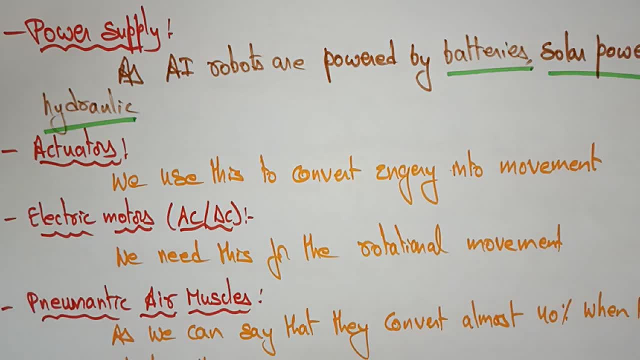 solar power and hydraulic. Now coming to the next component in the artificial intelligent robot that is activated. So what these activators will be used? We use these activators to convert the energy into moment. So everything the energy, if you are giving the suppose. let us take solar system. 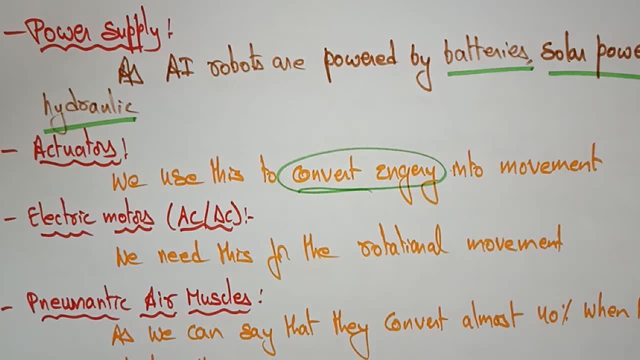 So whenever it is taking the energy- that is, a light energy from the sun- okay, and it is giving some hot water and it is going to do some moments- the electric bulbs is going means the bulbs are giving a lightning, Everything. because of this, some the heat energy, the heat energy is converted into the light energy. 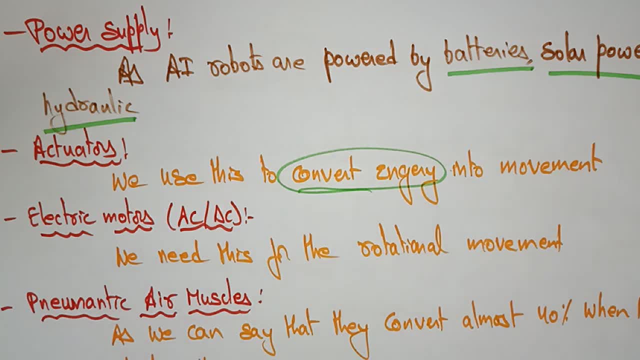 Okay, so like that, activators that are used in the artificial intelligent robots. here it is going to convert the energy. Okay, whatever the energy that we are giving in the form of a power supply, whatever it is that it is going into moment. Next component is electric motors. 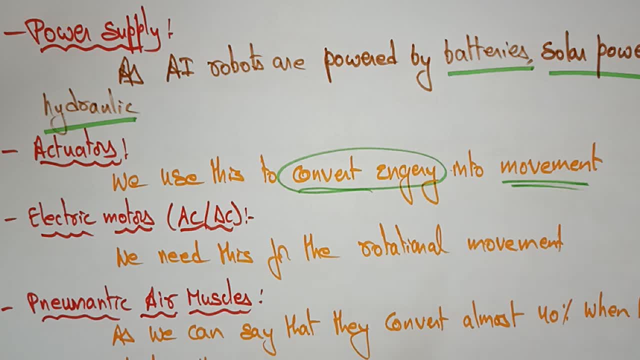 So here we used AC and the DC electric motors. We need this For the rotational movements. So why we use this electric motors? whenever the robot wants to move forward or backward or some rotations, everything that moments it has to perform means we need these electric motors with the help. 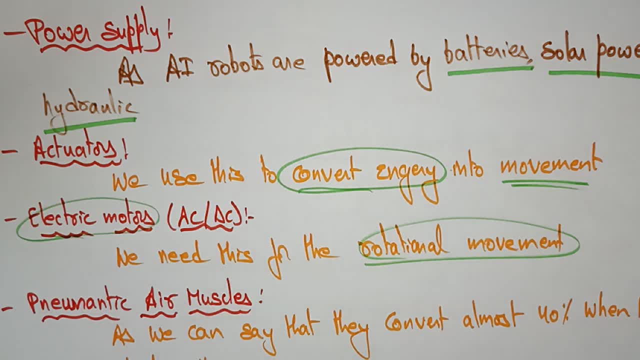 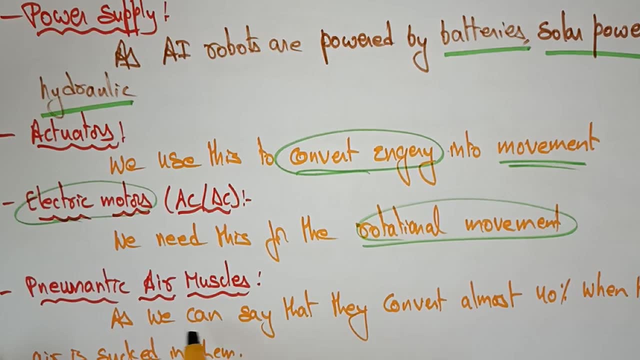 of electric motors only the system is going to move. Okay, for rotational movement, We are using the electric motors. next, pneumatic air muscles, as we can say that they can convert almost 40% when the air is circled in them. So how this will be worked. 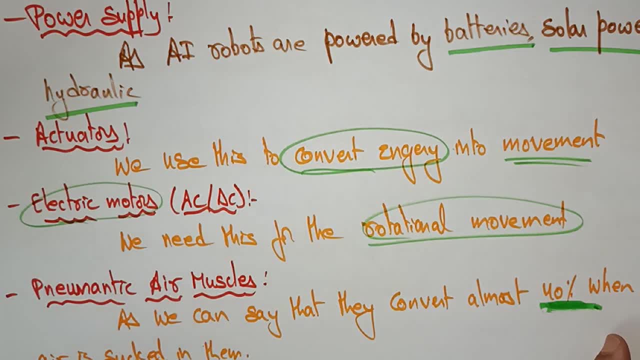 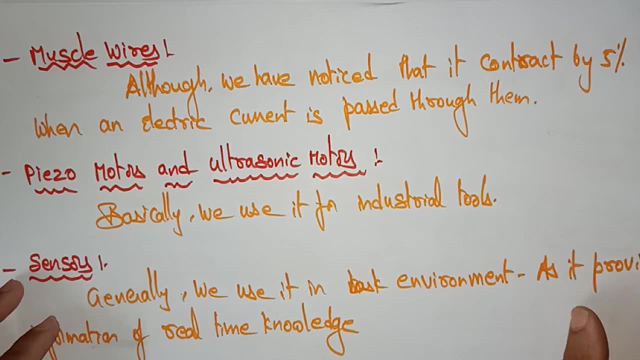 The air muscles eat whenever the air is circled in them. that is a almost a 40%. then it is going to be work. Next is the muscle wires, although we have noticed that it contrasts contract by 5% when an electric current is. 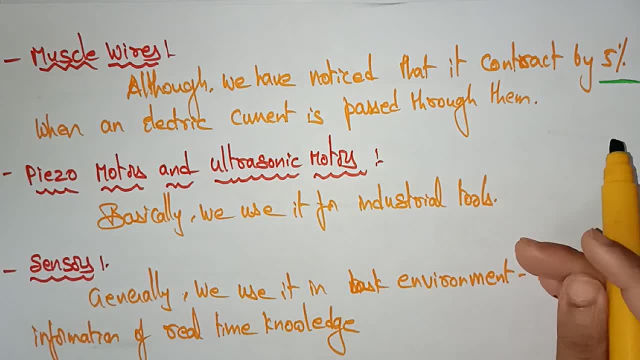 passed through them, then only this muscle wires is going to be work Okay at a power generation. electric current is passing through that wires, PSO motors and ultrasonic motors, actually these type of motors. Basically we use it for the industrial tools, only for the industrial tools. 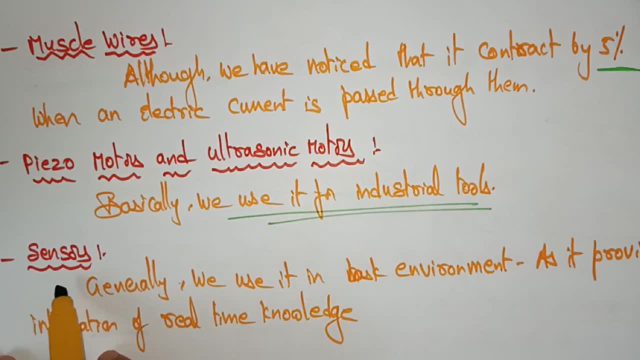 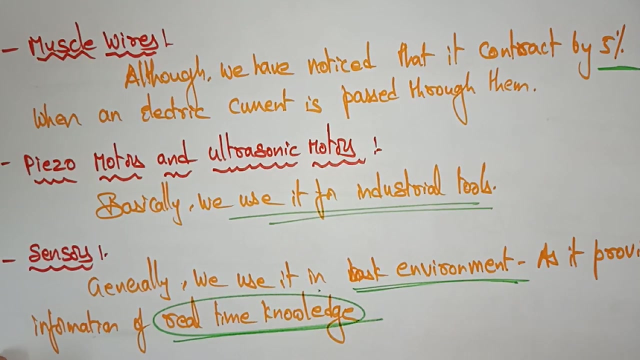 We will go for these type of motors in robot session. and coming to the sensors, So sensors is one of the important component that is in the artificial intelligent robot. Generally we use it in task environment as it provides information for real-time knowledge wherever we are working on a real-time knowledge. 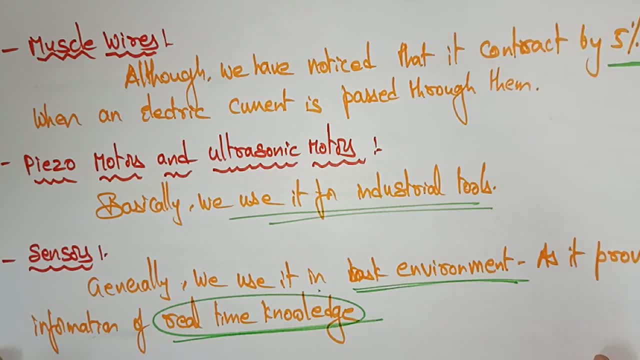 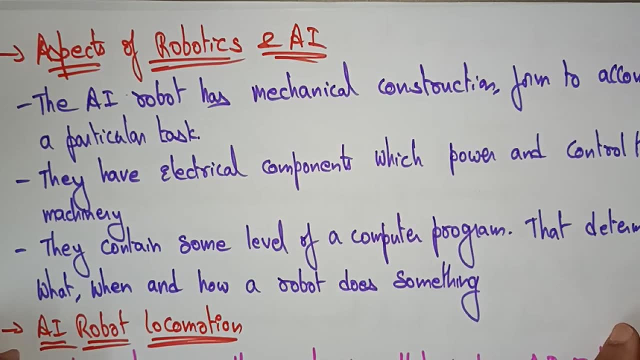 These sensors are playing a very important role in artificial intelligence. So these are all the different components of the artificial intelligent robots. Now let's see the aspects of robotics and artificial intelligence. So what are the aspects in robot when you talk about the robotics and when you talk about the artificial intelligence? 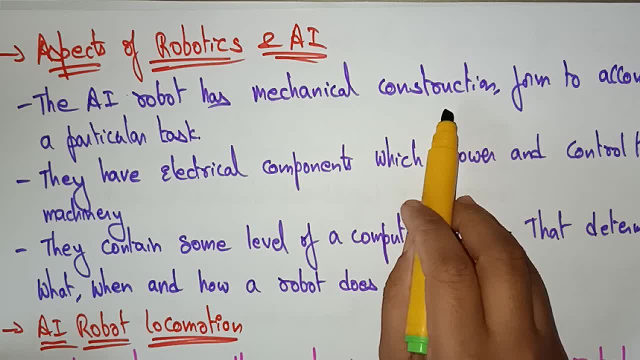 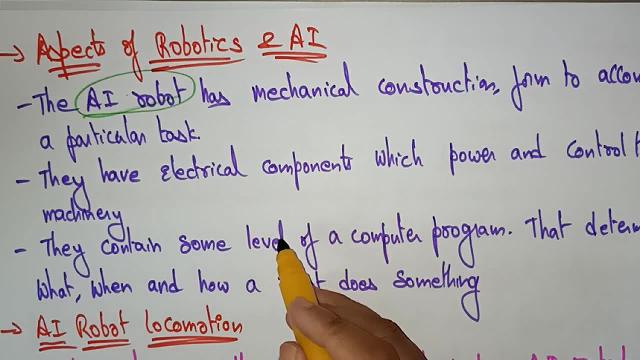 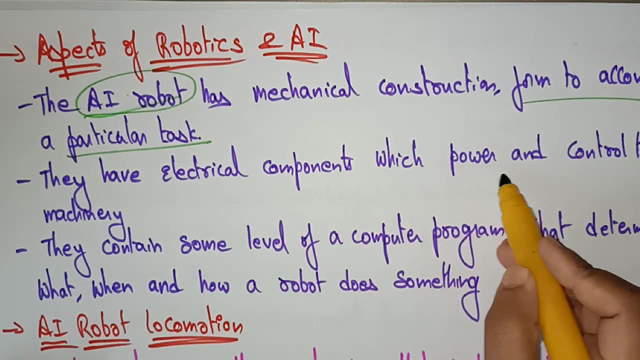 The artificial intelligent robot has mechanical constructions formed to accomplish a particular task. So what is artificial intelligent robots is doing? It is going to do some mechanical constructions which form to accomplish a particular task. They have electrical components which power and control the machinery also and they contain some level of computer programs. 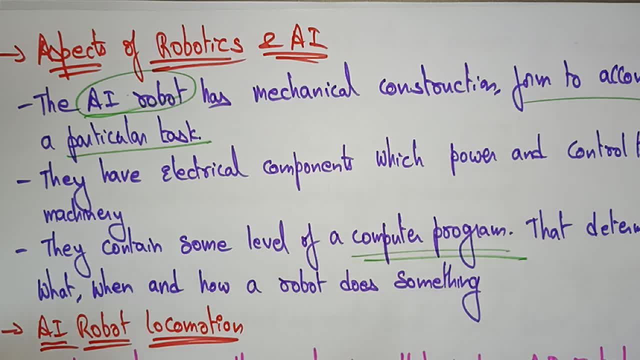 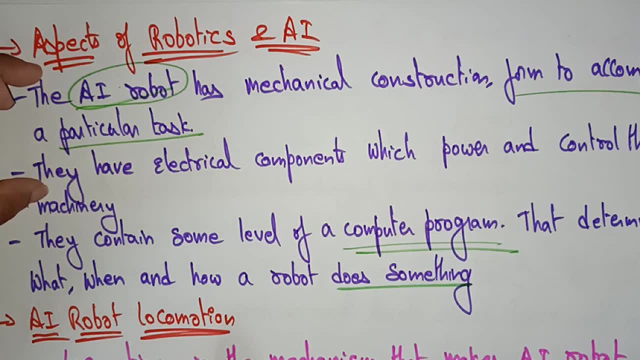 So this robotics and artificial intelligence contains some level of programs that determines what, when and how a robot does something. So what is this is going to be? do that the computer contains some level of programs, that that computer program is going to determine what, when and how a robot does something? 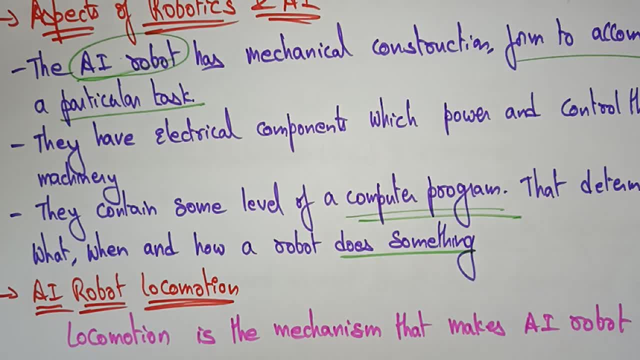 Now coming to another, That is a artificial intelligent robot: locomotion, locomotion, locomotion- the name itself It is a motion- means we are moving. motion is just a movement either. It can move how it is going to be moved. The locomotion means how it is going to move with the help of the legs or with the help of the wheel. 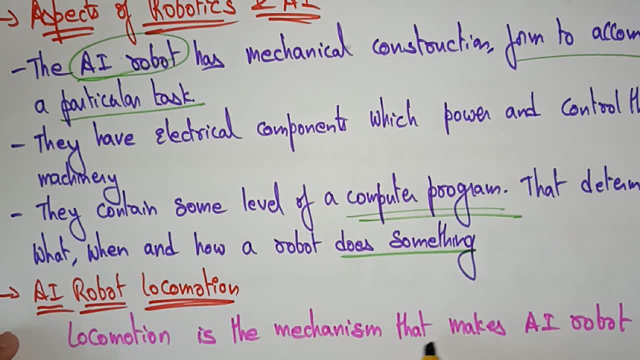 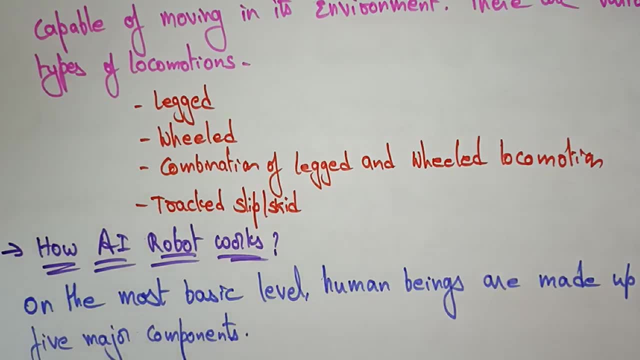 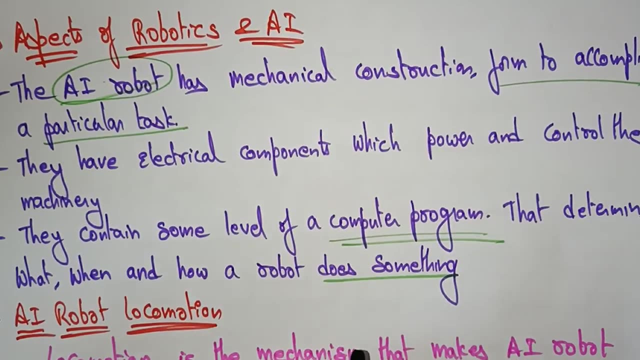 So how it is going to move. Let's see. the locomotion is a mechanism that makes artificial, intelligent robot capable of moving its own environment. So how, with the help of some technique, This locomotion, that is, the, the robot, is going to be move. 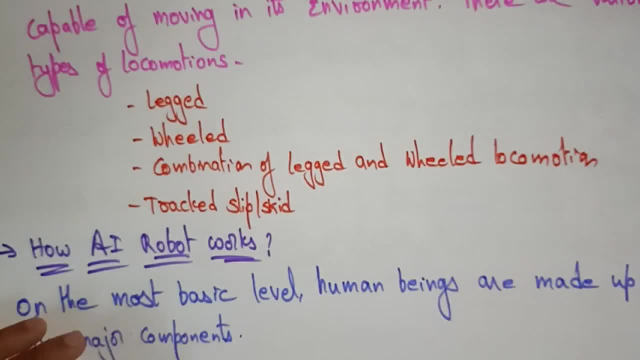 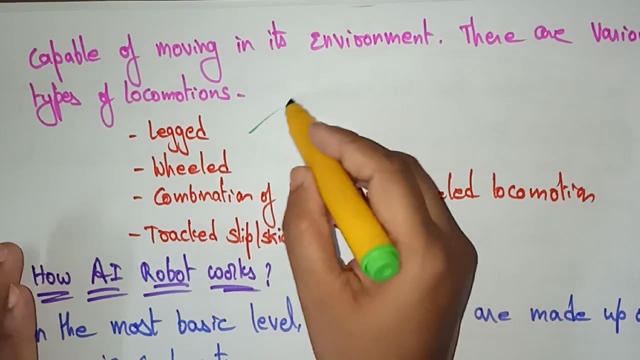 So locomotion is a mechanism that makes artificial, intelligent robot capable of moving in its environment. So there are some various types of locomotions or they're like like good wheel and something made, some machines or the combination of legs as well as the wheel: locomotion. 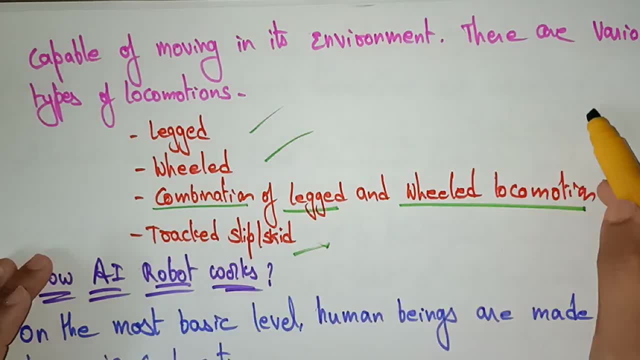 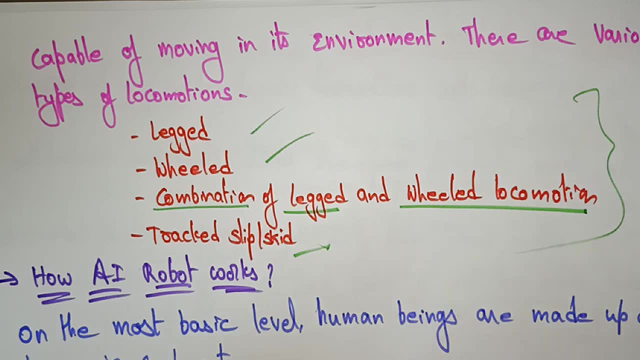 Also, and some track and slip or skate. So these are all that, with the help of these components, that the locomotion is a a, a, a, a, a a in robotics so like. it means you can see, a human can keep an artificial leg. okay, so which is? 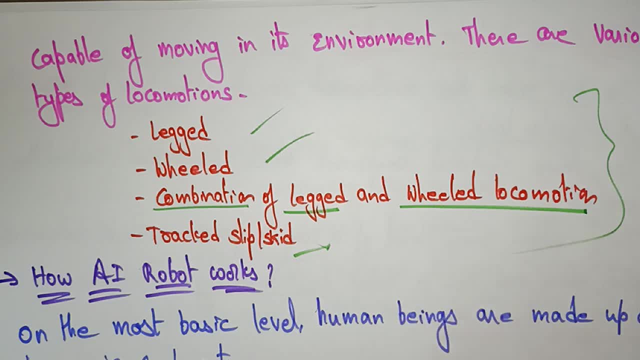 everything will be activators, everything will be installed and then it is moving just like a human. okay, it's a moving up and down, running, jumping, something. everything is doing. then coming to the wheel type of robots: a wheel is attached to the robot so that it will be rotate and move forward. 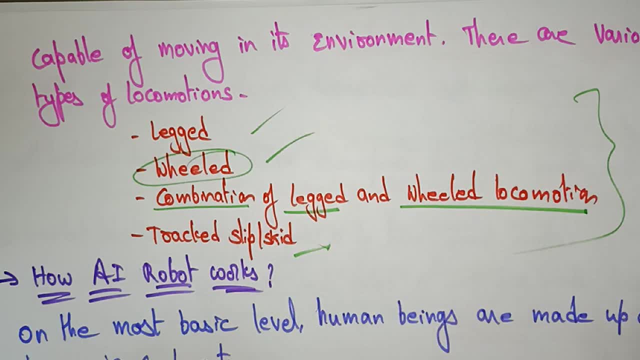 and move backward and it rotates the wheel. but legged means in whatever the direction you can go- you can go right and you can go left, you can jump and you can see everything you can do- but in coming to the wheel type of robots, it only rotates and it will go forward or it will go backwards. a robot- 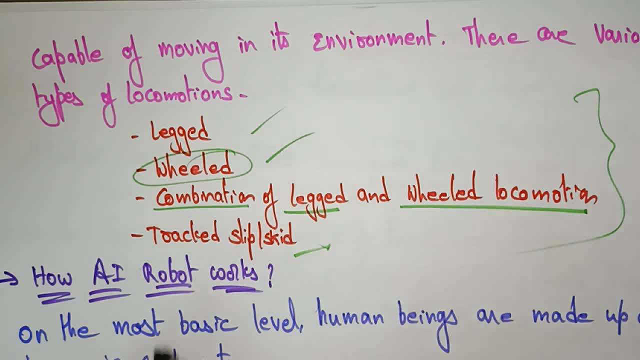 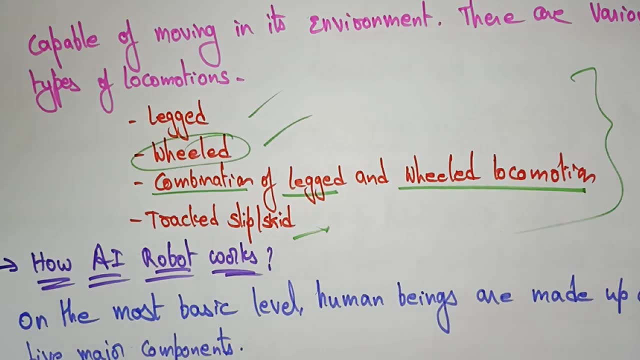 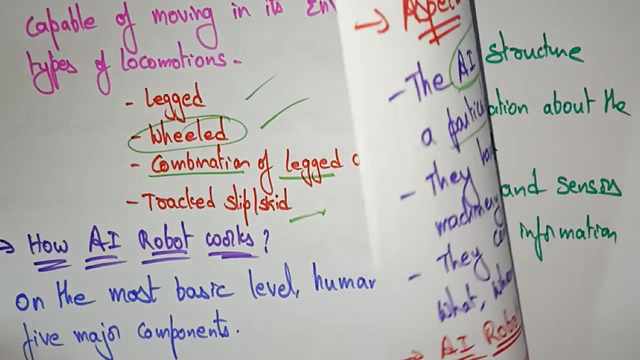 the legs will be like wheels. they are wheels or keeping, otherwise it should be a leg. sometimes it is a combination of legged and wheel. both will be there. so how artificial, intelligent robot works. on the most basic level, human beings are made up of five major components. 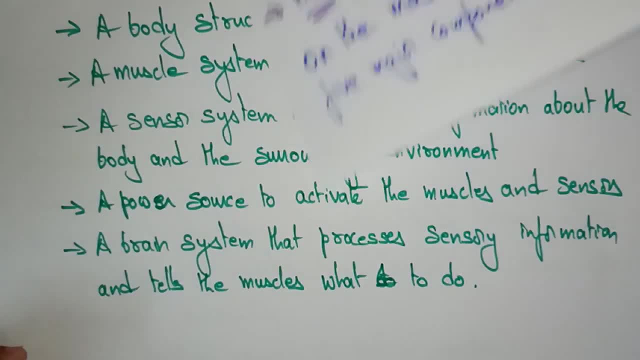 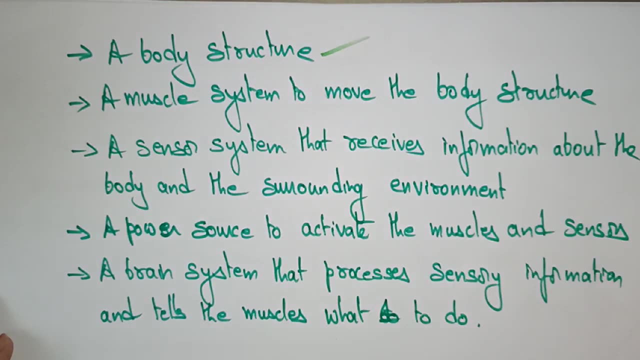 based on these only, the artificial intelligent robot is also work because it's just like a human. the robot is acting just like a human, so it is also having the body structure, a muscle system to move the body structure. so actually human is having these five major components: a body,